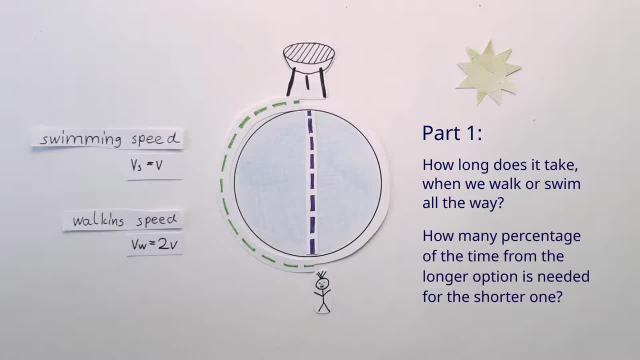 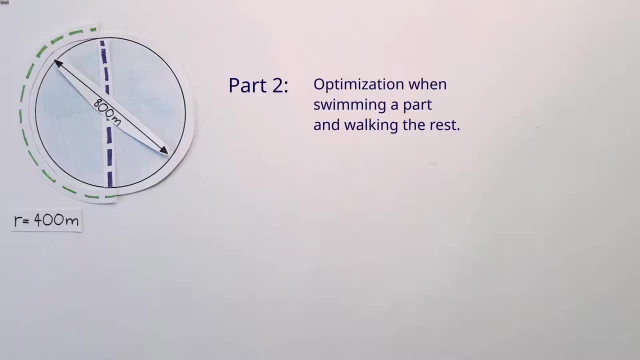 In addition, we will calculate how many percentage of the time from the longer option we would need for the shorter one. In the second part of this video we will check whether we are faster if we swim one bit and then walk the remaining part. For the time calculation we need the distance and the speed, So T-swim equals distance. 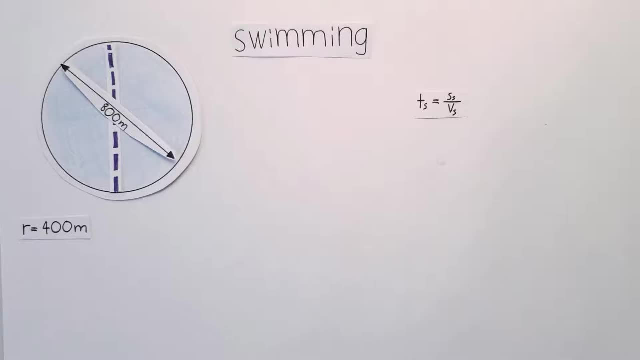 swim divided by velocity swim. The same applies to the walking. Additionally, we know that we are walking twice as fast as swimming, So V-swim equals V and V-walk equals to 2V. Next we have to calculate distances. We swim across the lake, So the swim distance 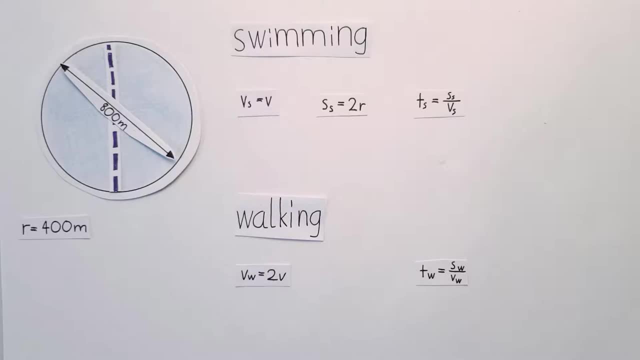 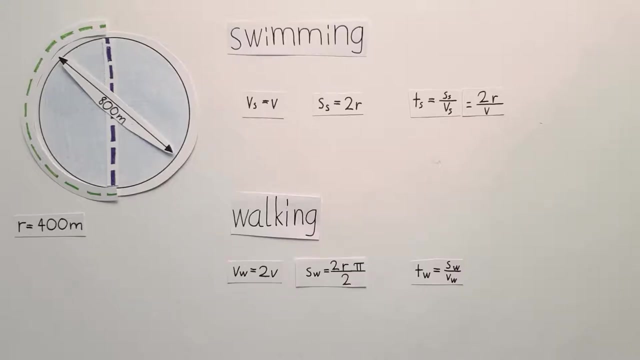 assass equals to 2R. Now we can insert everything into Ts and get 2 times R divided by V. Now to the walk distance. The circumference of circled is 2Rpi, But as we only walk around half the lake, We only need half a. 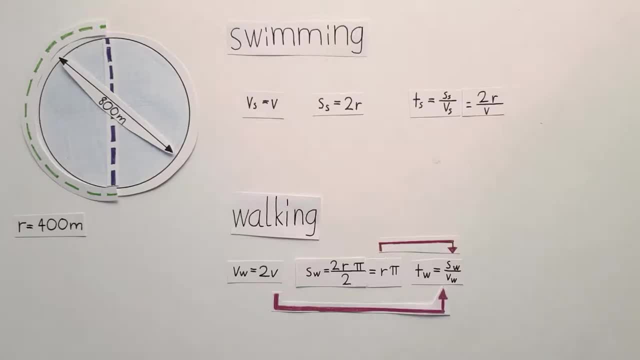 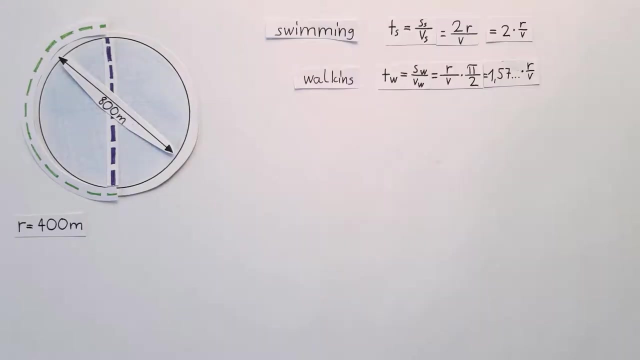 of it Again. we can insert this into the time formula twalk. Now we rearrange it, which gives us r, pi divided by 2v. Calculated, we get 1.57 times r divided by v. That's less than swimming. For swimming, we need 2r divided by v, Although we don't know the absolute. 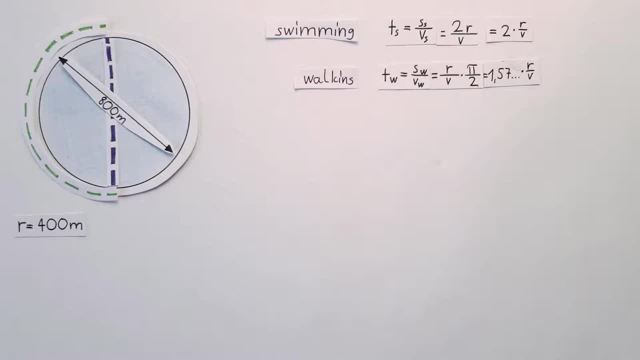 time. we know it, depending on the radius and the swimming speed, v Swimming is the longer option and therefore 100%. Now, what percentage of the swim time is the walking time? The formula for calculating the percentage is p. percent equals part divided by whole. For us this means time walk. 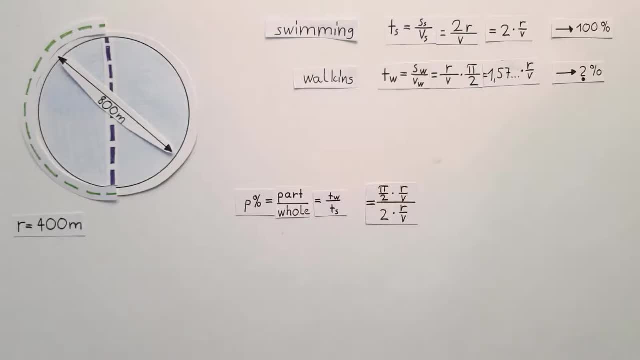 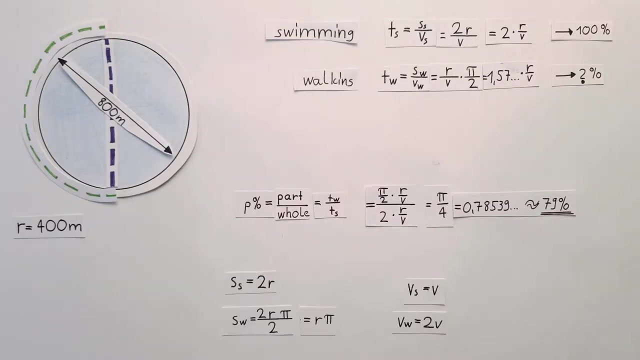 divided by time: swim. Next we insert the formulas and reduce. That gives us pi divided by 4, which equals 79 percent. So walking takes only 79 percent of the time needed for swimming. Actually, the way to walk is exactly pi half long To. 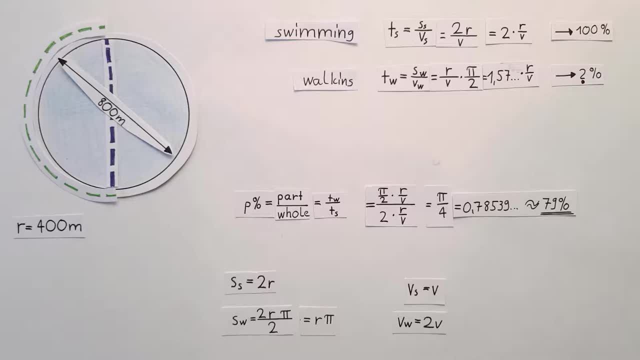 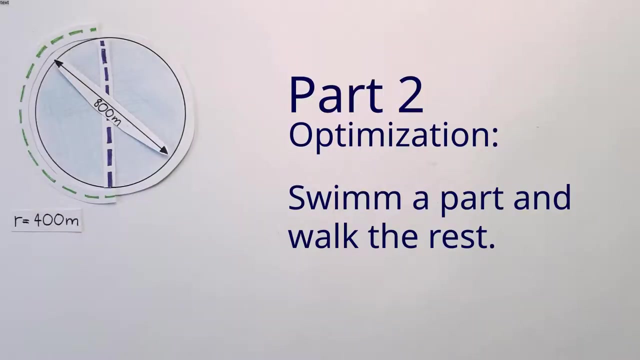 be as fast as swimming. the runner must be exactly pi half faster, which is about 1.57.. But we walk two times the swimming speed, so we are faster with walking. In the second part we will account for the calculate with radians. This will simplify the calculation and make it easier for us. 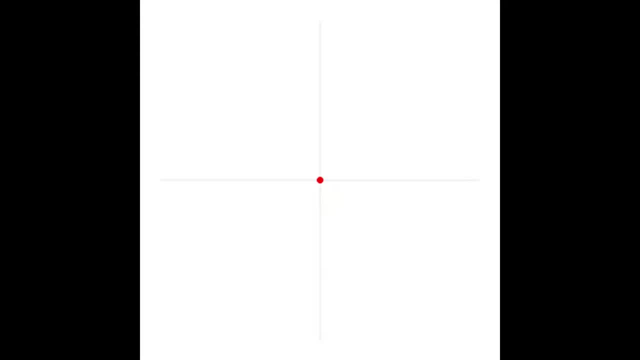 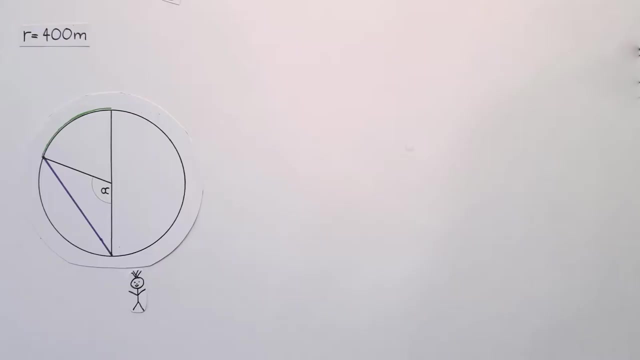 As a short refresher, this animation explains the radians in a nutshell. That's the unit circle with the radius equals to 1.. Now to the task. We are currently at point A and want to go to point B on the opposite side of this lake, as soon as possible. 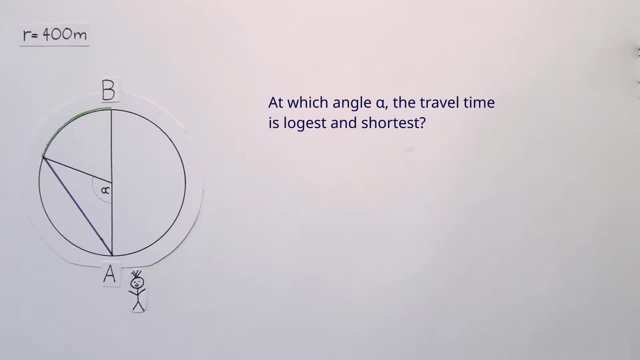 The options of walking or swimming have already been discussed in the first part, But now we can also swim a part for our task, For example up to point P, and then walk the rest along the lake. The ratio between swimming and walking is determined by the angle alpha. 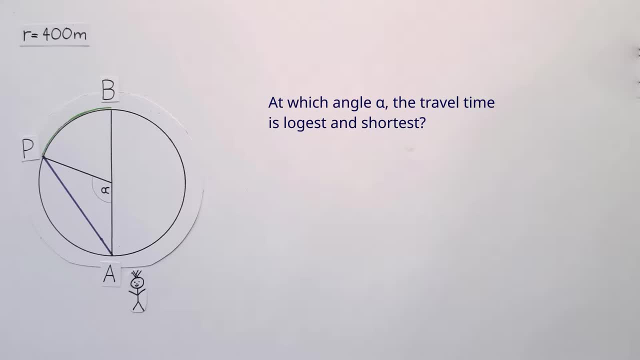 Alpha describes the angle from A to the midpoint, to P. So the distance we want to swim, The distance which we are going to walk, is described by pi minus alpha. This because in radians, pi equals to 180 degrees. We will calculate the swim time as well as the walk time as a function of alpha. 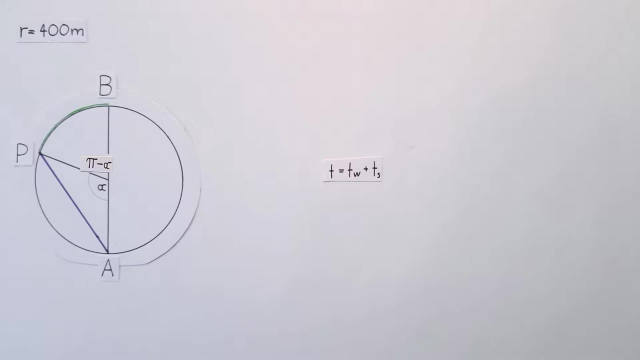 Then we will sum them up to get the total time needed. This formula will then be optimized. So let's start with the walking distance. Many of you may have heard of the formula for the walking distance. Many of you know the formula for the arc length in degrees. 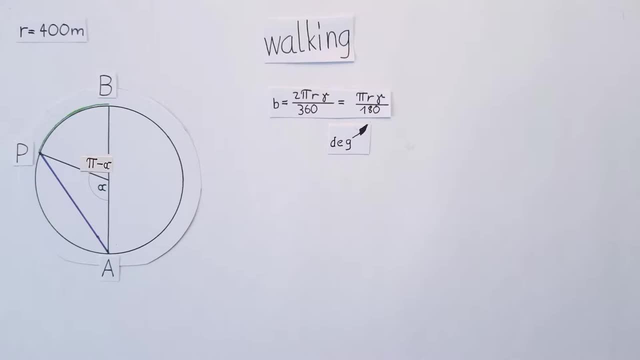 Pi times r times the angle in degrees divided by 180.. We will therefore proceed on the basis of this formula. We replace 180 with pi and then reduce. Thus you get the arc length in radians, r times the angle in radians. But our angle for walking is not gamma, but pi minus alpha. 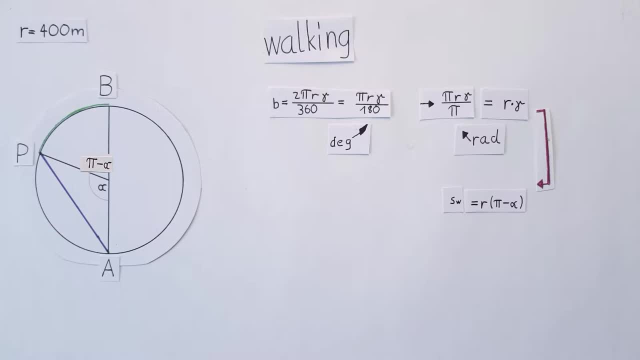 And so we already have the walking distance. The walking speed is still 2v. Also, the walking time equals still walking distance divided by walking speed. Therefore we insert this into the formula and multiply it Now to the swimming distance. Imagine we cut out the triangle A to the midpoint P. 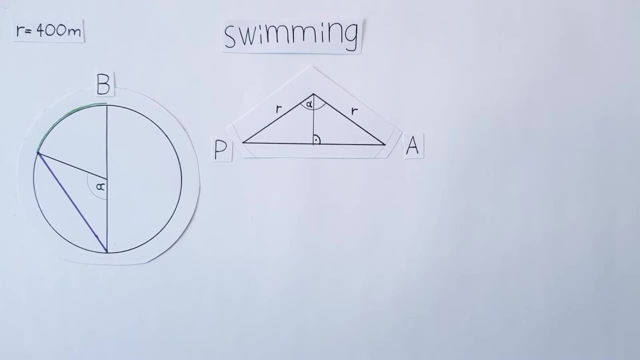 This is not a right angled triangle and therefore it's difficult to calculate the side as S. But we can cut the triangle in half In order to calculate half of the swimming distance. We know the hypotenuse r and the angle alpha half. 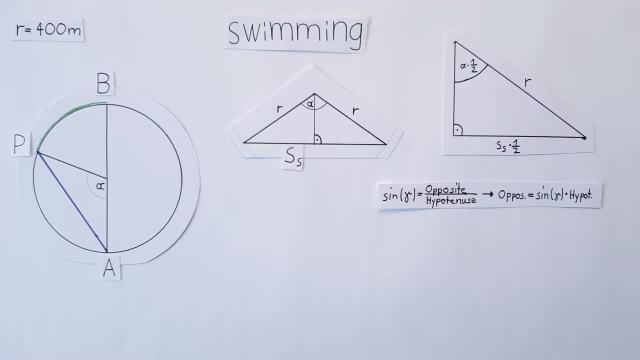 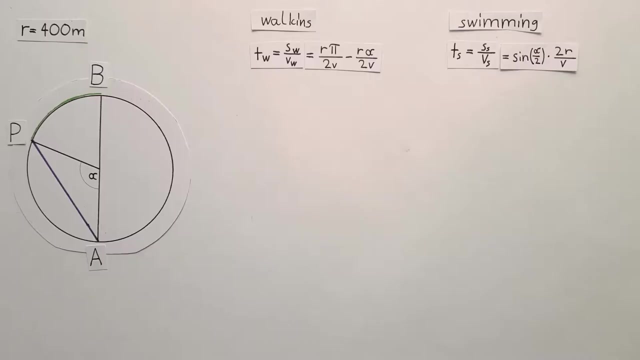 Ss half is the opposite. Therefore, Ss equals sine of alpha half times r times 2.. Otherwise we would only calculate Ss half. Speed and time calculation are still the same. Therefore we can insert and get the swimming time. So finally we have everything we need to calculate the total time in dependency of alpha. 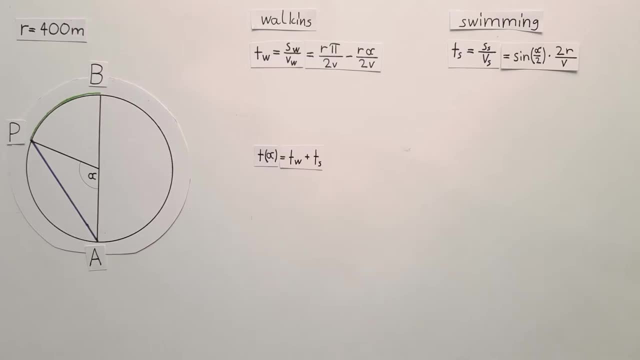 t equals walking time plus swimming time. So let's insert that We want to keep the time as short as possible. Therefore we want to optimize t. To do so we have to take the derivative and then find the zeros. The derivative of the first two summands are zero and minus r divided by 2v. 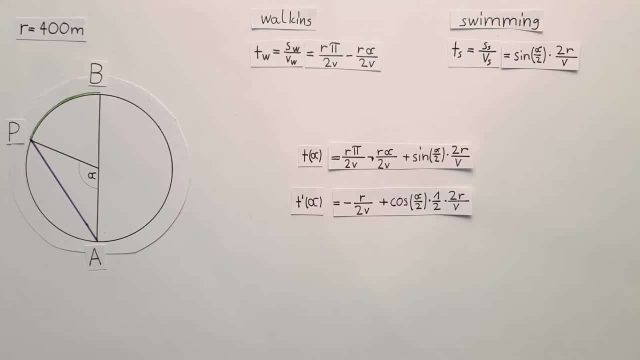 For the sine we need to apply the chain rule. The derivative of sine is cosine. Alpha half stays in the cosine, But the derivative of alpha half is one half and then, multiplied r divided by v is a constant and can be left as it is. 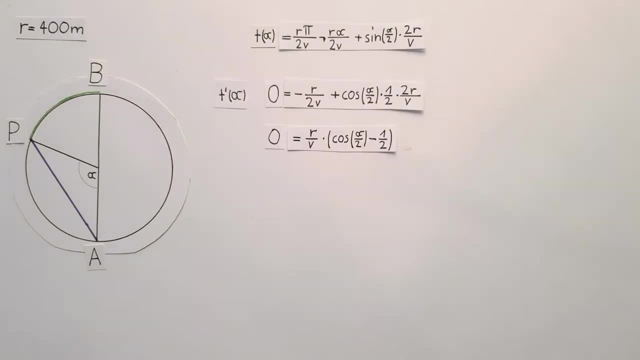 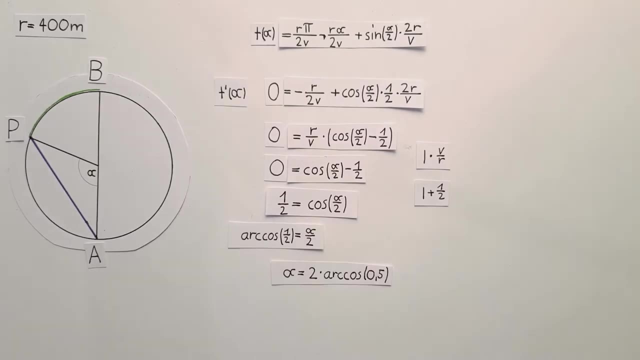 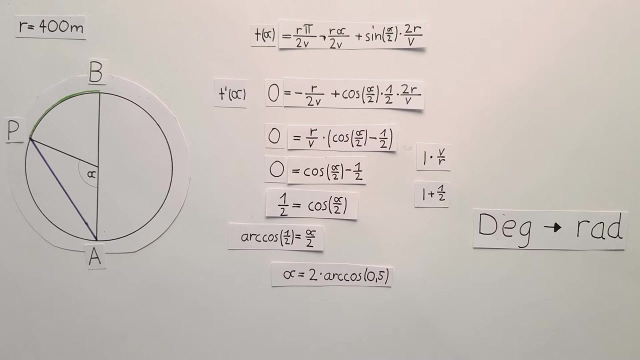 Now we have to find the zeros. We solve the equation to alpha. After several steps we arrive at: alpha is 2 times arc cosine of 0.5.. At this point, Don't forget to change your calculator from degrees to radians, Otherwise the result is useless. 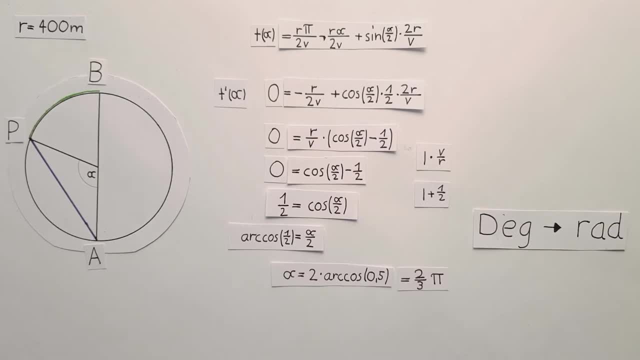 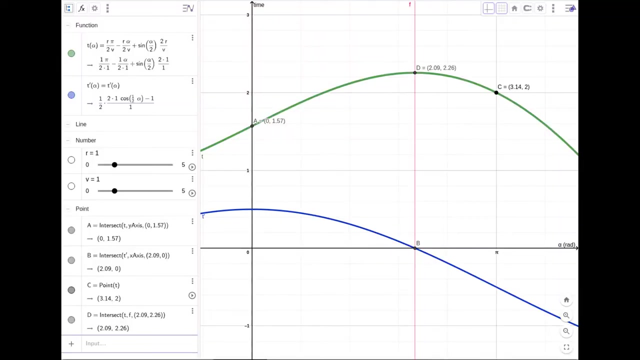 That gives us 2 third pi, which equals 120 degrees. So finally, we found the minimum. Well, are we sure about it? Let's check the graphic device. We are only interested in the range from 0 to pi. Green is the function and blue the derivative. 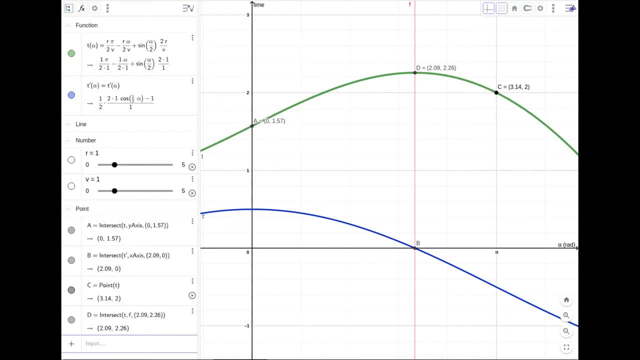 At point A, alpha equals 0 and correspondence as if we walk all the way. For this we need pi half time, as we calculated in the first part. At point C we swim the whole distance because alpha equals 2 pi. For this we need the time of 2.. 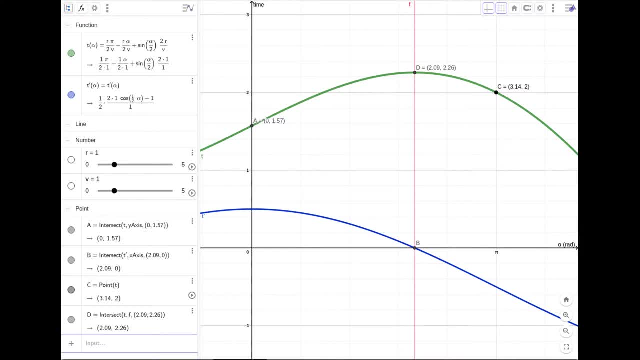 Also this we have been calculating in the first part. D is our optimized time, But it's not a minimum, it's a maximum. That means we reach our friends fastest when we walk around the lake. Just swimming is not the slowest, but not as fast as walking.